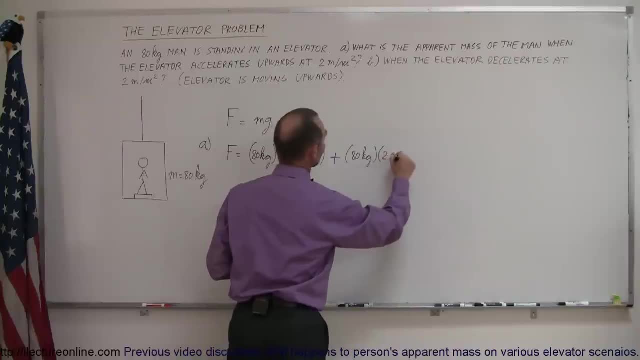 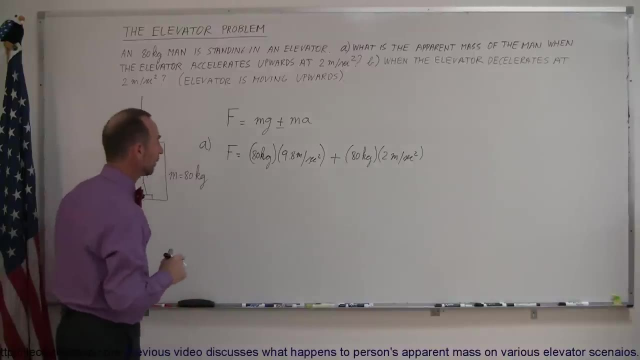 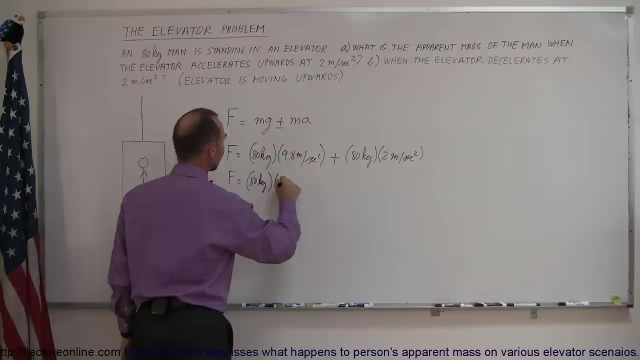 that would be an elevator. but actually acceleration is two meters per second squared, so that would be the additional weight pushing down on the on the scale. so the total force is equal to 80 kilograms times 9.8 meters per second squared, plus 2 meters per second squared. so we factor out in 80 kilograms and then with a calculator let's see. 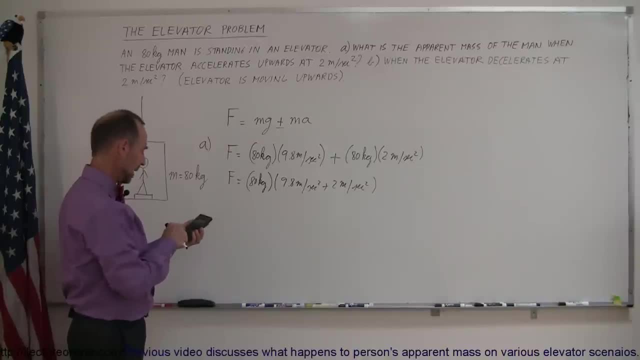 what that is. so the force would be 80 times the quantity 9.8 plus 2, and that would be 944 newtons. okay, so what is the weight? that is the weight of the person on the scale, but what is the apparent mass? and so, since we know that the weight, the force, is equal to the mass of the man plus the, 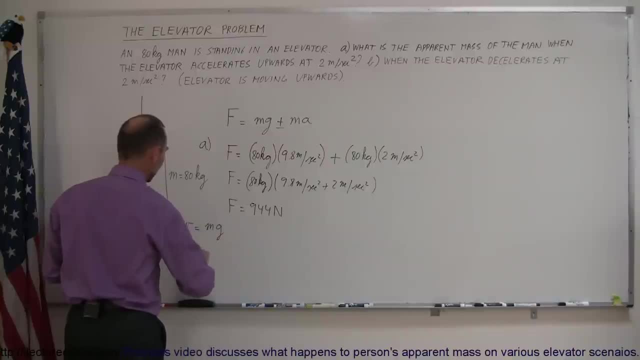 force is equal to weight, which is equal to mg, then that means that the mass is equal to the weight divided by g, which in this case is the force divided by g, which is equal to 944 newtons divided by 9.8 meters per second squared. and if we divide this by 9.8, we get 96 kilograms. 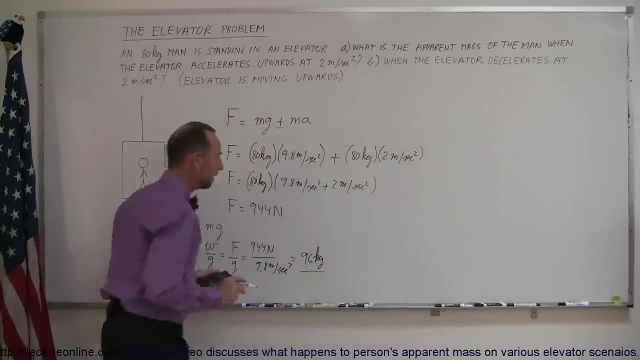 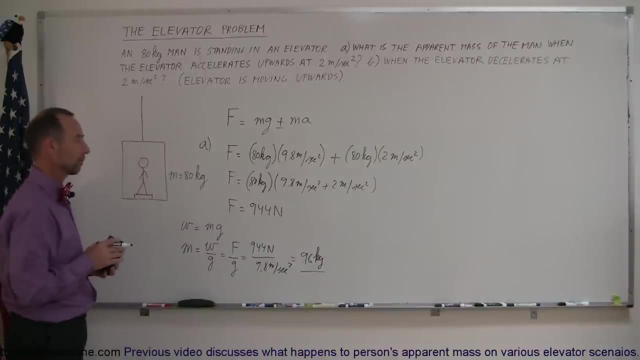 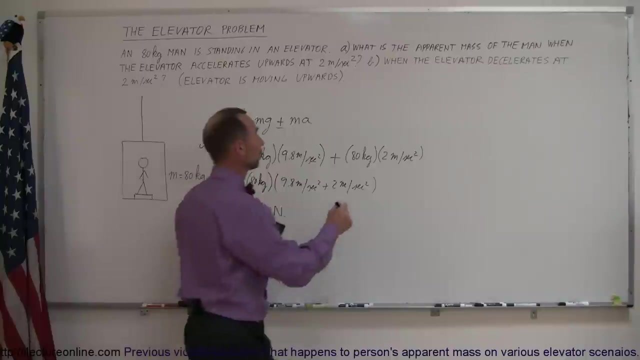 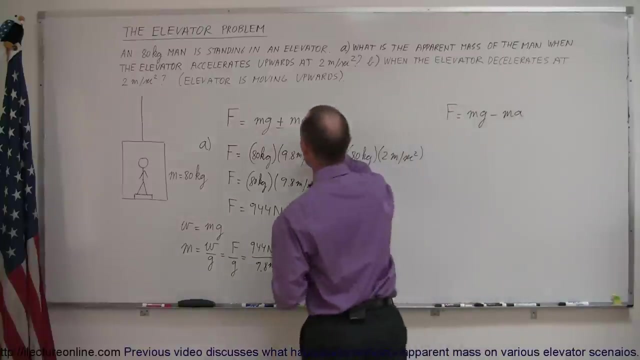 so we can see that the scale as the elevators moving upward would show 96 kilograms instead of 80 kilograms. now what would happen when elevator reaches the floor the person wants to get off on and the elevator begins to slow down. so there's a negative acceleration. so at that point we have: the force is equal to mg minus ma. so remember here: 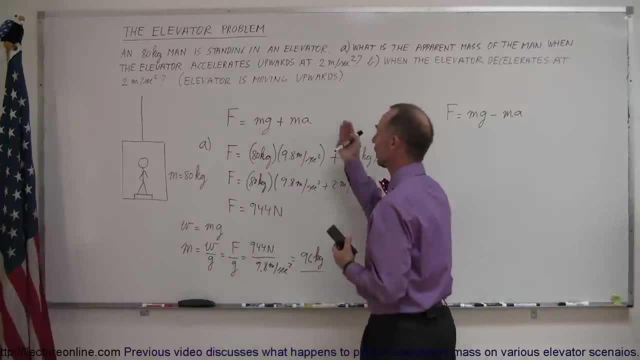 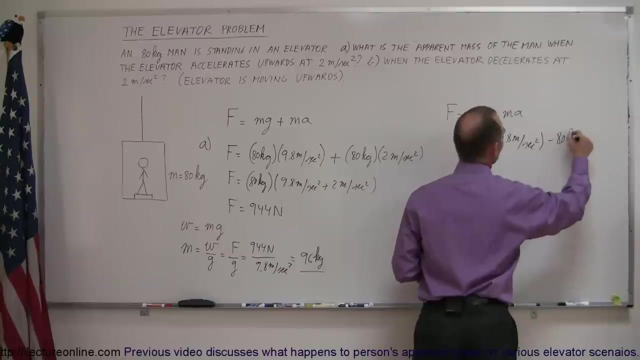 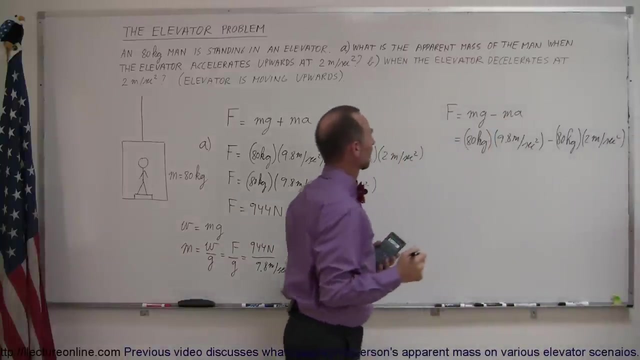 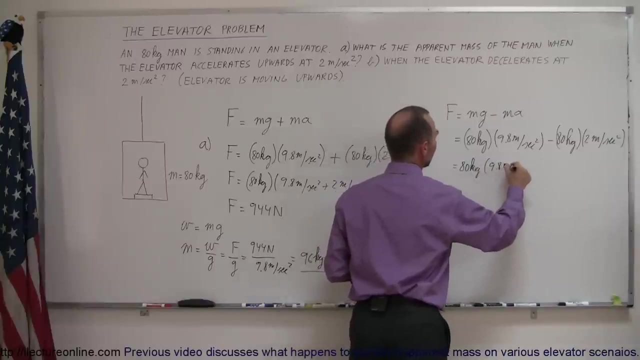 that we got rid of the minus, because we're accelerating upward here. it's minus goes for accelerating downward. so this is equal to 80 kilograms times 9.8 meters per second squared, minus 80 kilograms times 2 meters per second square. so this is equal to 80 kilograms times 9.8 meters per second squared, minus 2 meters per.